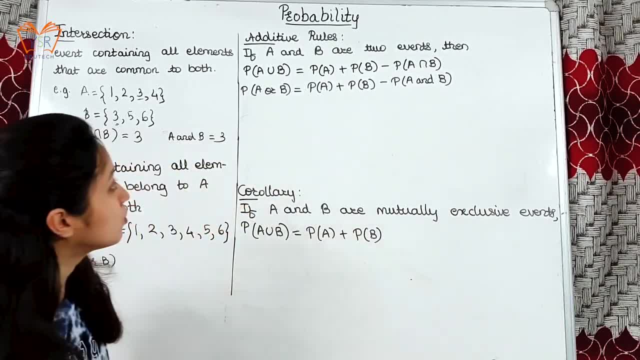 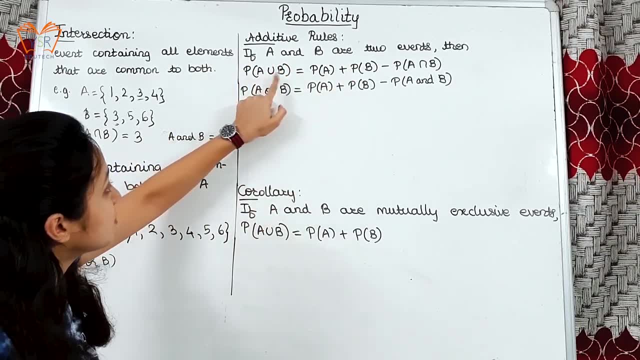 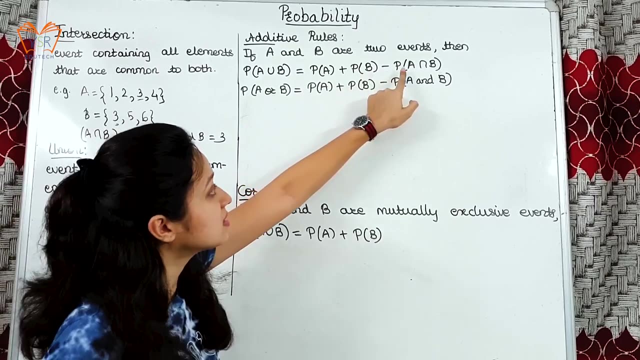 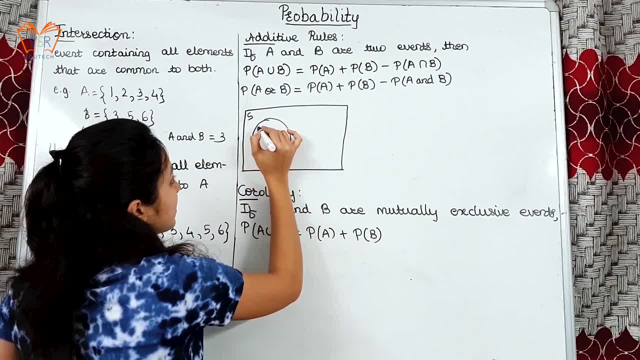 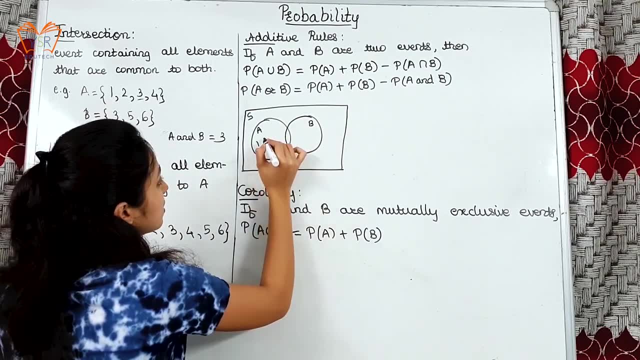 with this problem. So let us start with this problem. So let us start with this problem. space S and we have event A and event B. We will take the same example: 1,, 2,, 4,, 5,, 6 and. 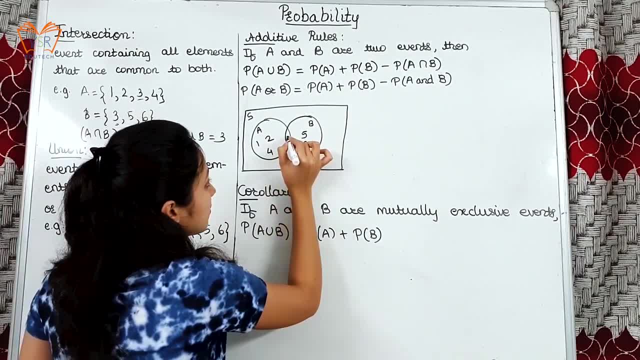 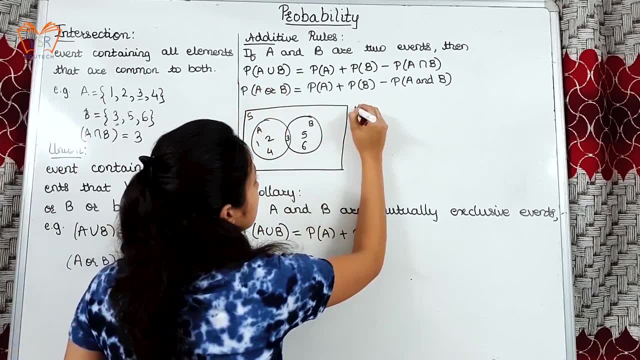 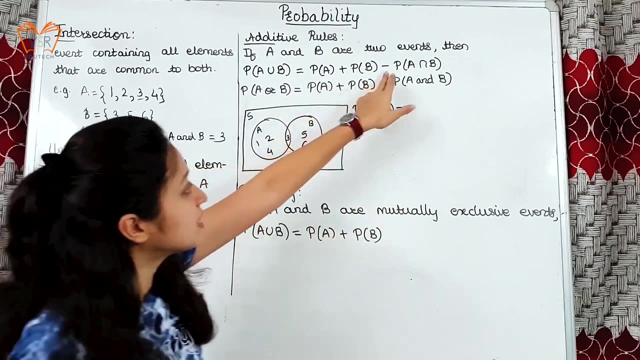 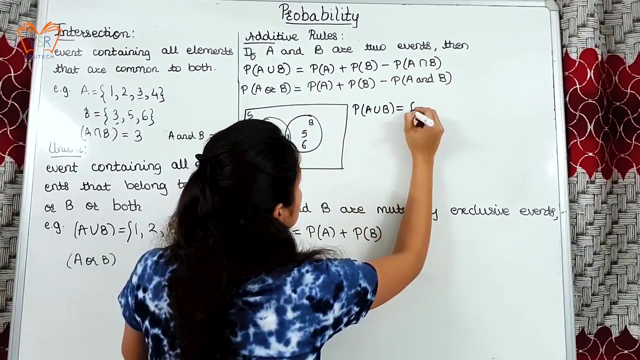 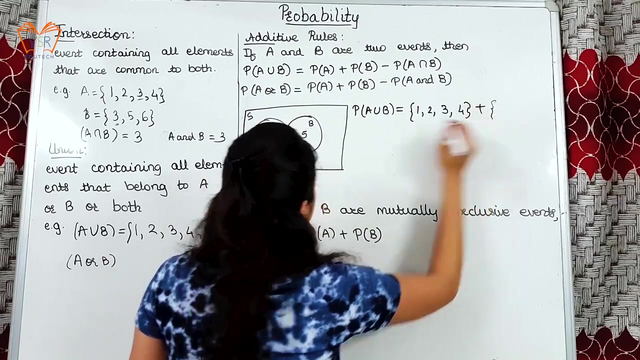 as we know, 3 is common between both, So 3 will be written here, That is, it is included in A as well as in B. Now union will be. Now, why do we need to subtract the intersection of both? That means suppose now, the probability here is 1, 2,, 3, 4 plus 3, 5, 6.. 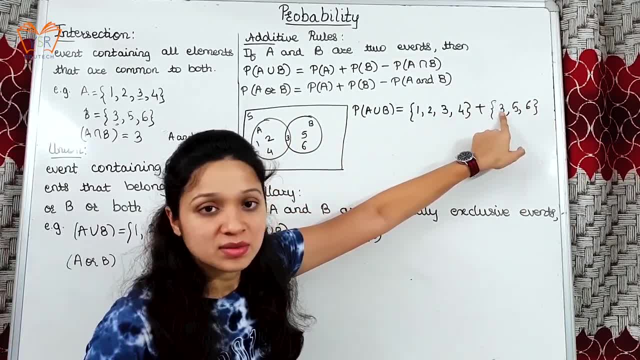 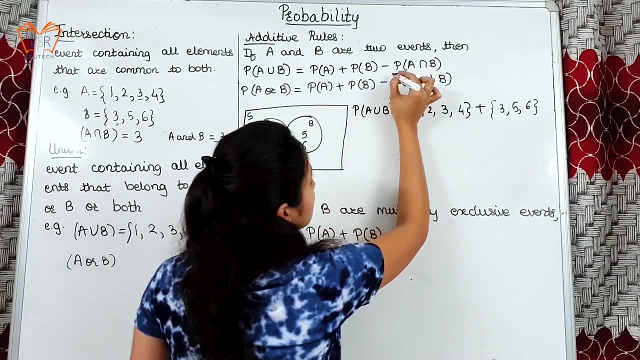 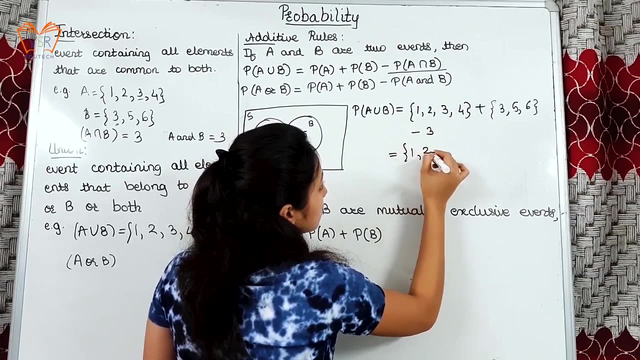 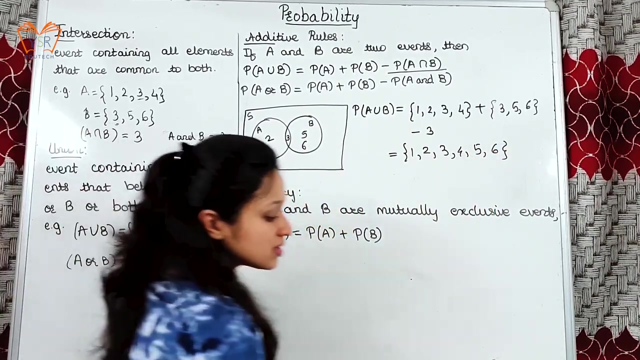 Now, if you see, 3 comes twice, but in the union we need 3 only once. So to subtract this common element, once we are including this term, that is intersection of both the events. So minus 3 will give us total 1, 2, 3, 4, 5, 6.. Now this is about the two events, A and B. If we 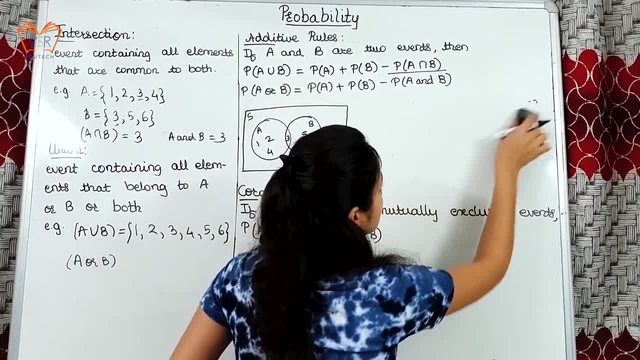 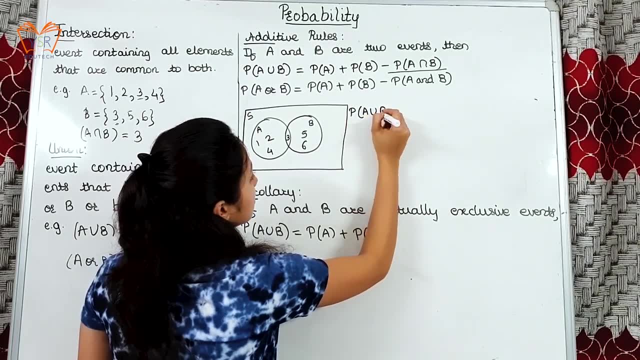 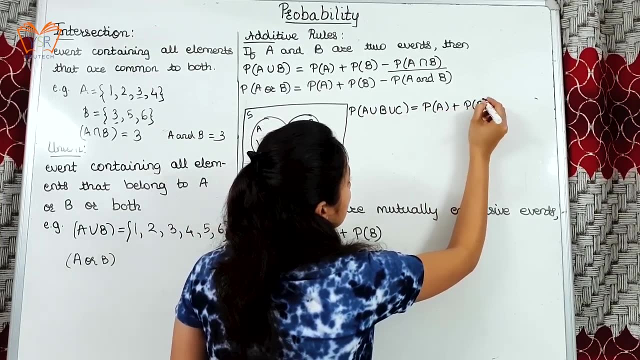 extend this formula for 3,, 2,, 3, 4 plus 3,, 5,, 6.. Now, if we extend this formula for 3, the events: it will be A, union B, union C. Probability of each events. that is probability. 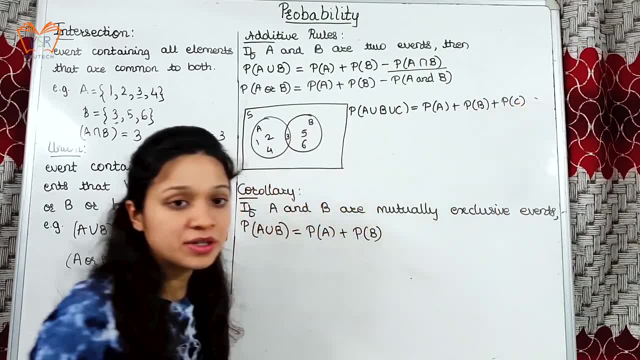 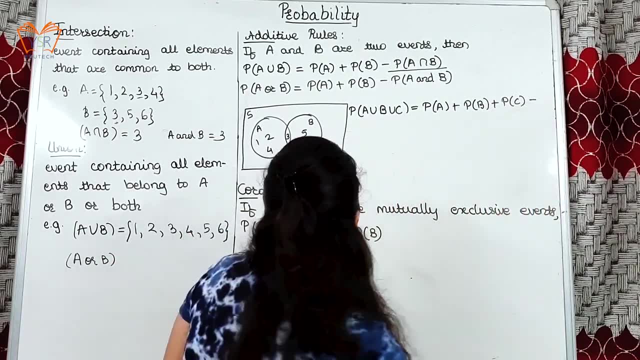 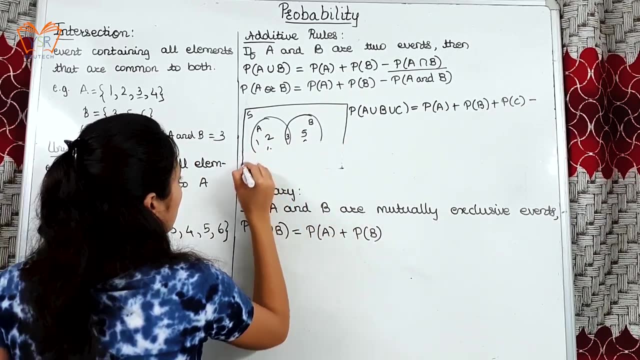 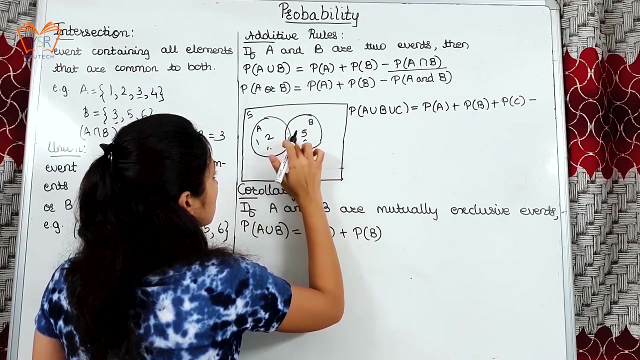 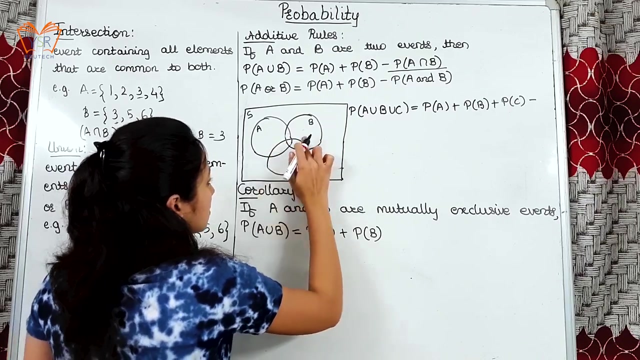 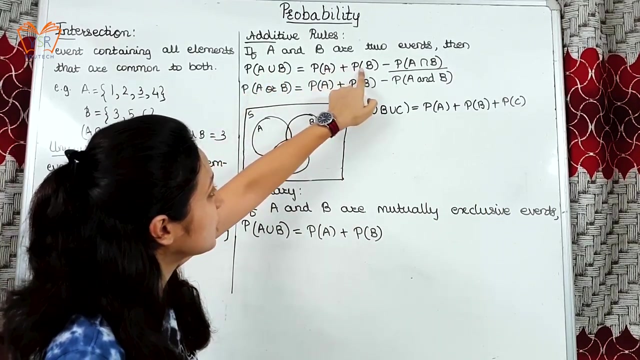 of event A, probability of event B and probability of event C. Now we are supposed to subtract the intersection Now. before that we will modify the Venn diagram and understand. So, As seen in the above formula for union, we are supposed to add the sum of individual. 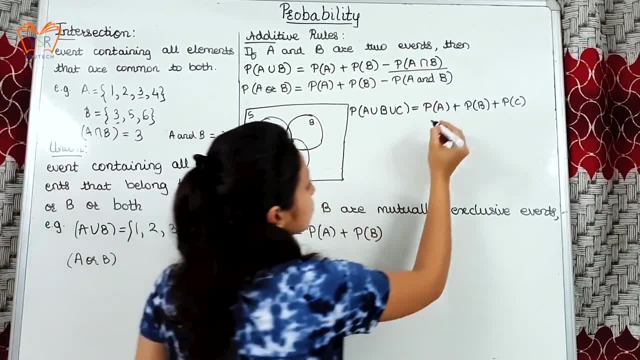 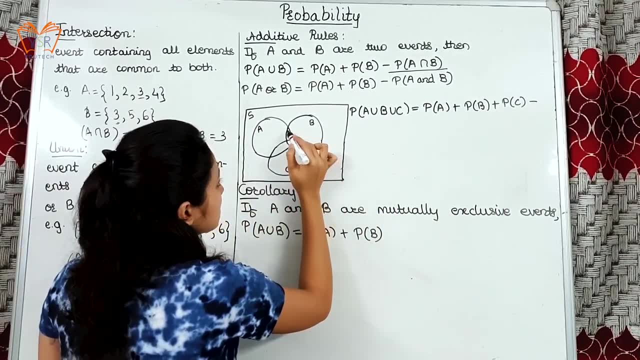 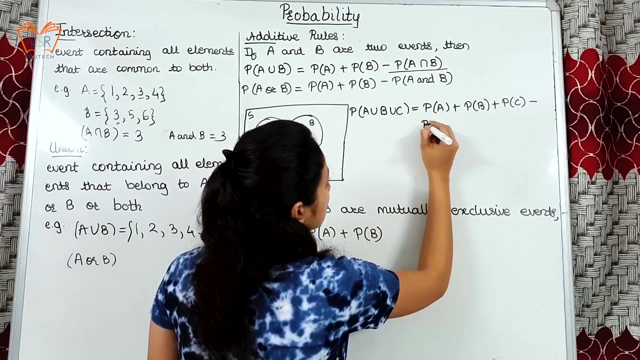 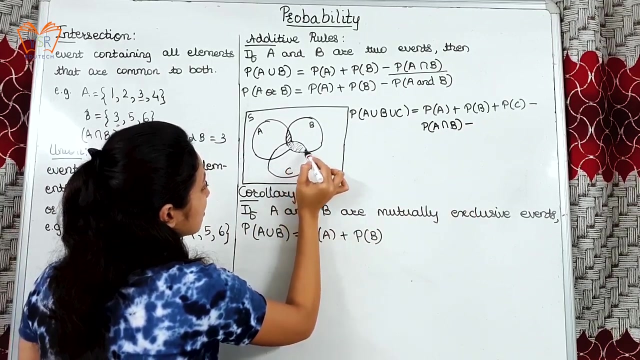 probabilities and then subtract the common elements. So this is the addition of individual probabilities. Now let us start subtracting the common elements. So if you see, this part entire is common in events A and B, so that will be subtracted. P, A, intersection B, minus again we have this part that is common in events B and C and 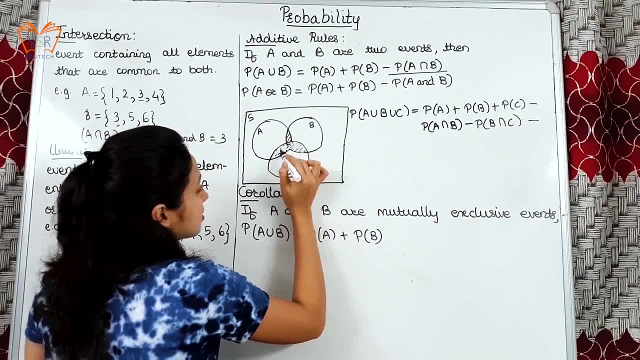 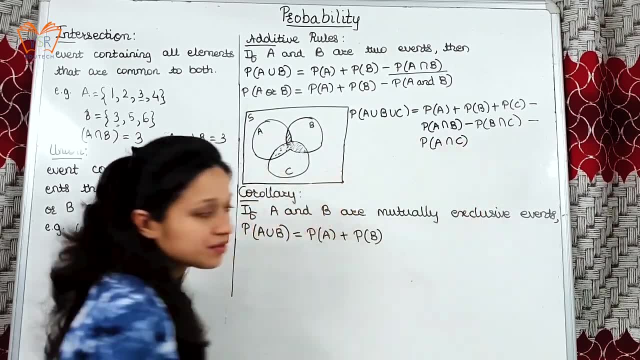 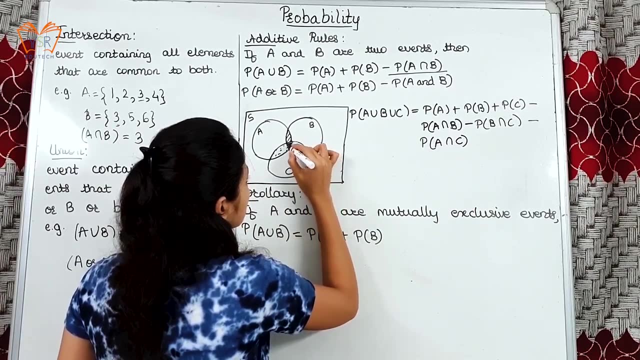 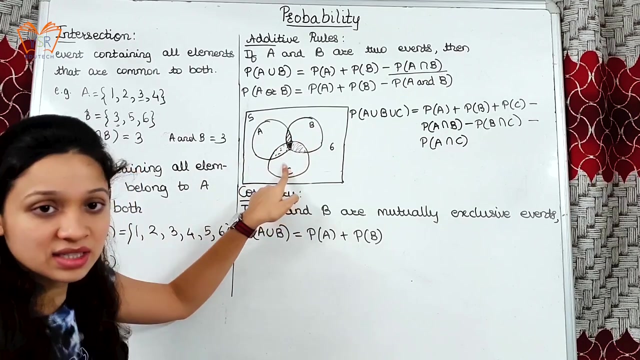 at the last. this is the part, So probability of event A, intersection event C. Now, if you see this part, suppose this part consists of element 6, that is common for all the events A, B and C, But that is getting cancelled because of the intersection part. 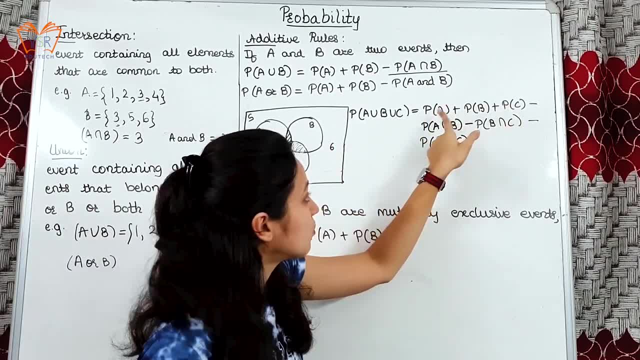 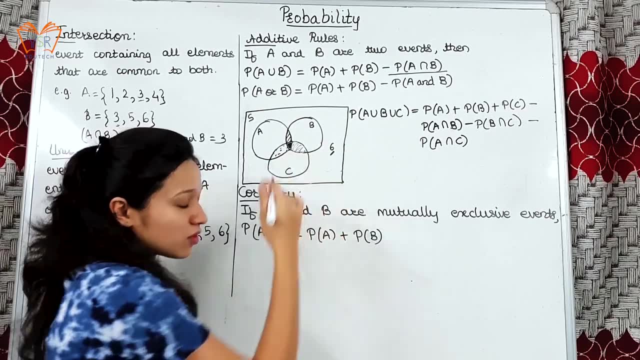 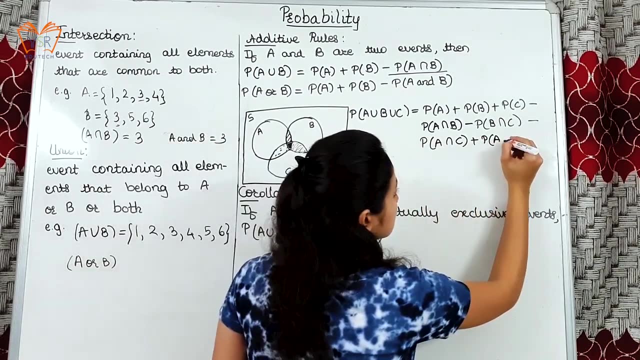 This 6 will appear thrice here in the addition of all the events, But will be subtracted in the intersection. So for the event, so for the element to appear at least once, we need to add the common element of all the three events, that is, A, intersection B, intersection C. What you do is you simply 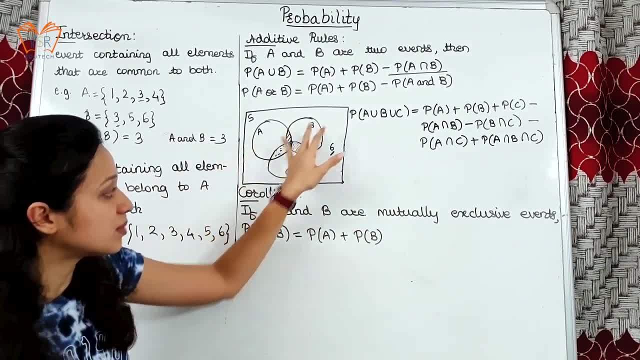 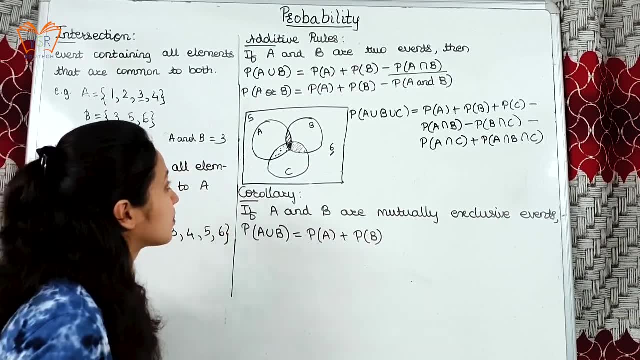 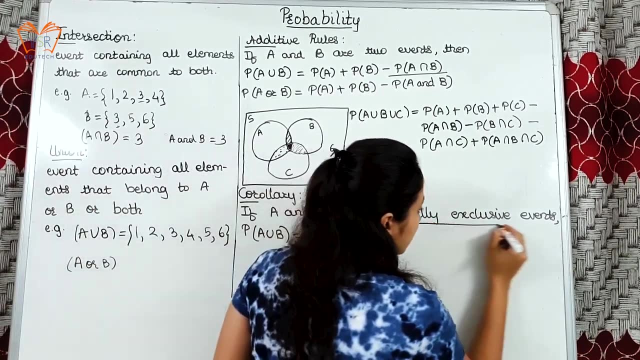 take an example that consists of various elements for A, B and C. Solve using this formula and see if you get correct. If you still have doubt, you can ask in the comment section Now if A and B are mutually exclusive events. Now, mutually exclusive events are those events whose intersection is equal to 0 or nullable. 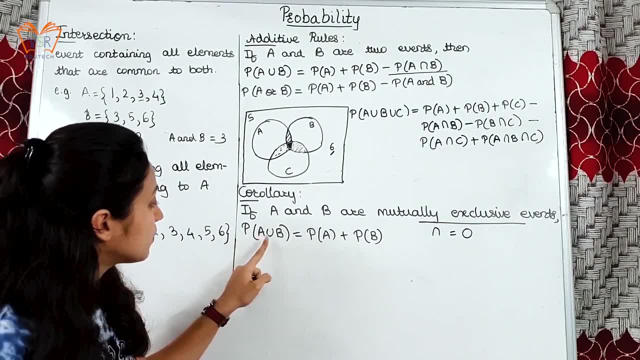 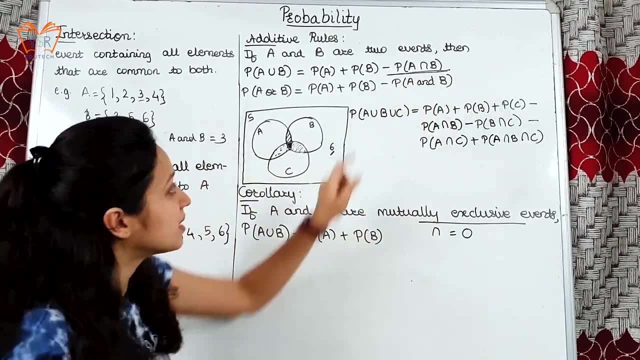 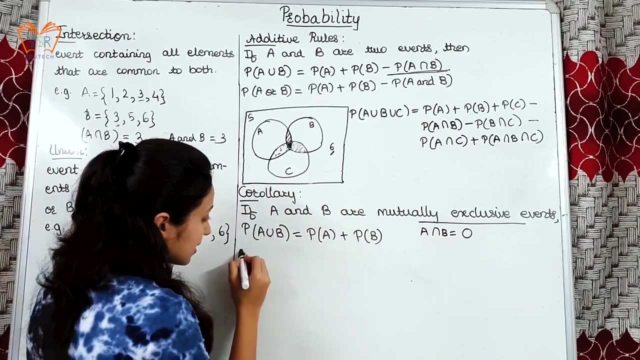 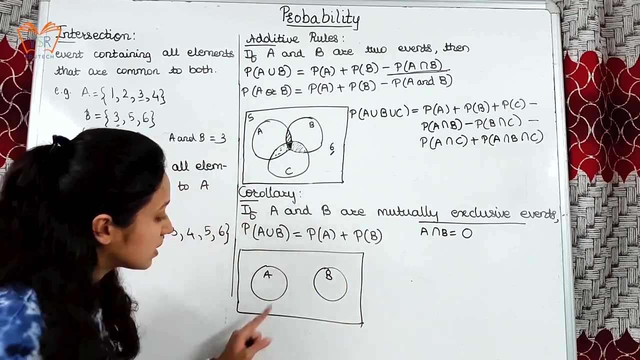 So the above formula will be modified as probability of union of two events is equal to sum of the individual probabilities and will not have the third term because anyway intersection is equal to 0. So Venn diagram can be modified as suppose this is event A and this is event B. They are. 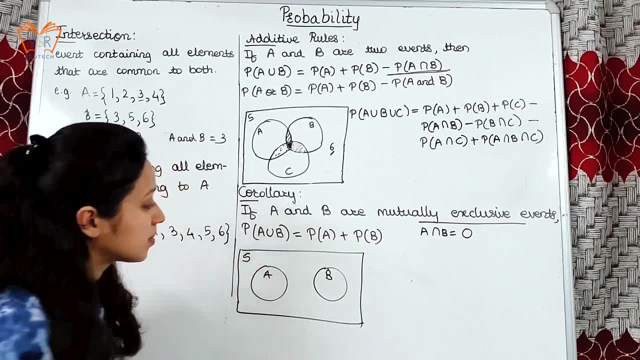 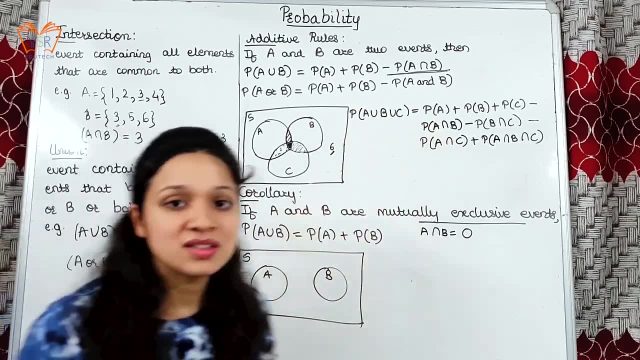 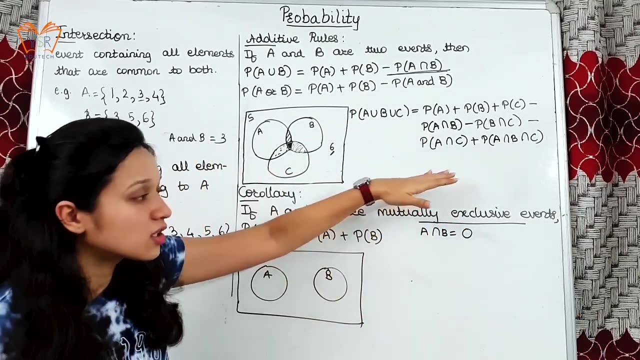 having no elements in common. Similarly, this formula can be written for the three events as well. This is task for you. Let me know the answers in the comment section Before we end. in last video, we studied complementary event and mutually exclusive event. This is task for you. 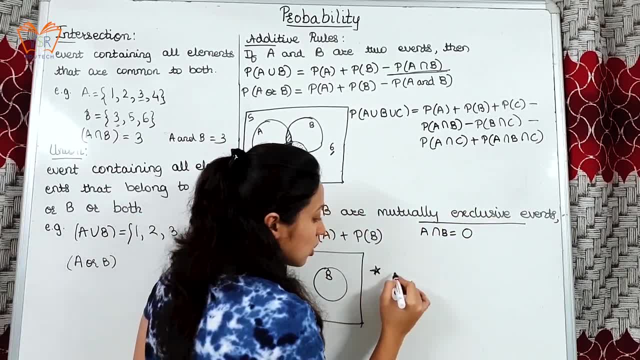 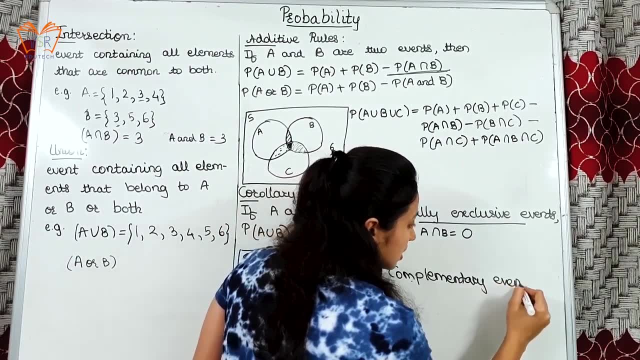 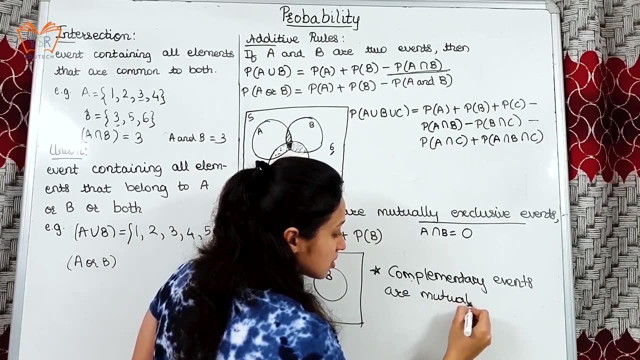 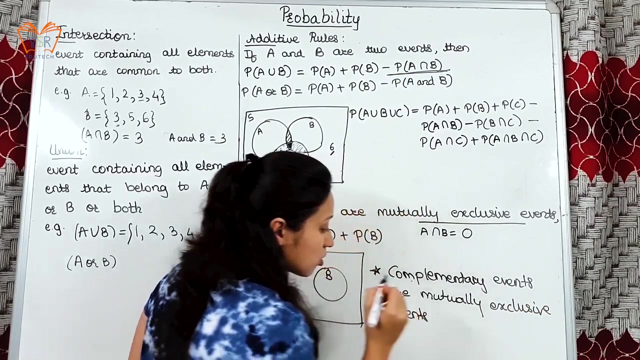 Let me know the answers in the comment section Before we end. in last video we studied complementary event and mutually exclusive event. There is an important note that all the complementary events are always mutually exclusive events, But the contrary is not true, that is, all the mutually exclusive events may or may not be. 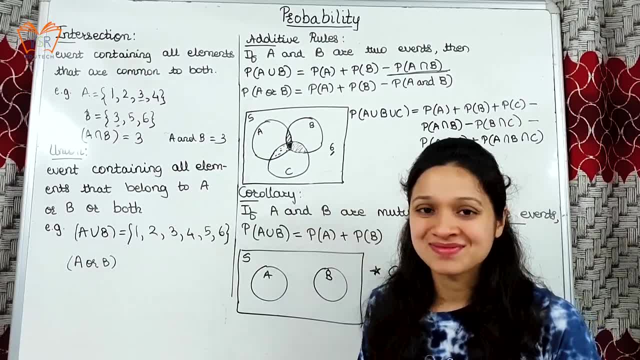 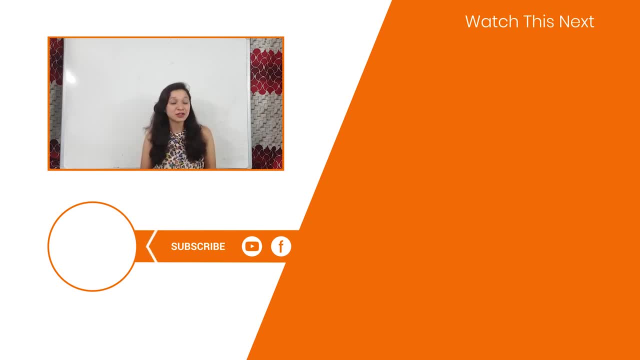 complementary events. Hope you understood, understood, thank you. thank you for your support till now. we need it for the tools, so please like the video, share with your friends and don't forget to subscribe to our channel, thank you.